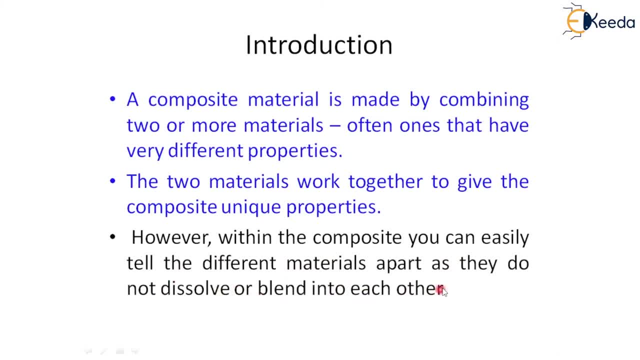 dissolve or blend into each other. this is the condition for a composite material. suppose, if you want to say any material as a composite material, so those two materials cannot have any chemical reaction, cannot dissolve or blend into each other, then only we can say that the material is a composite material. so here you can see what is exactly the various materials. 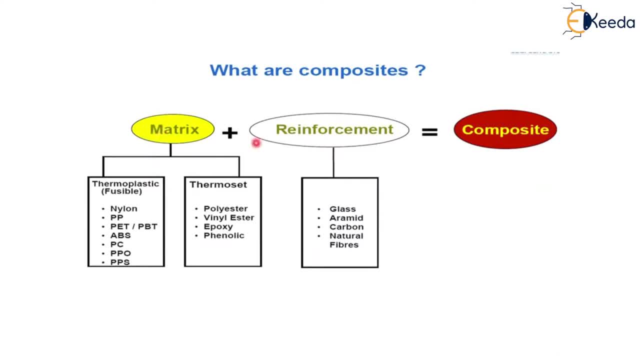 which are involved in composite materials. see two components we are seeing as a composite materials. first one we are representing as a matrix means the maximum percentage of the material and the second material we are representing as the reinforcement. together we are representing as a composite see under matrix. so many materials comes under that is it may be. 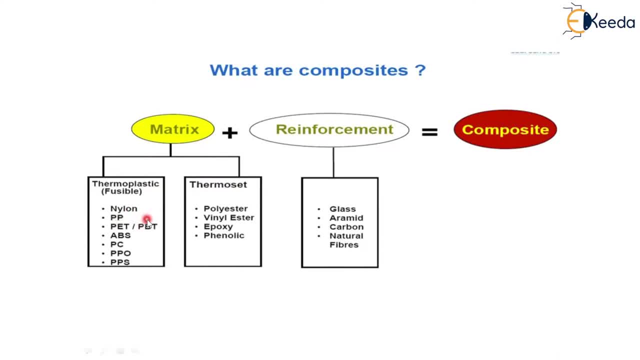 thermoplastic or thermosets. maybe nylon and here abs. so many materials comes under thermoplastic and under thermosets. polyester, vinylister, epoxy, phenolics- so many materials comes under thermoset. all these are under matrix. that means we are replacing these two materials as a maximum. 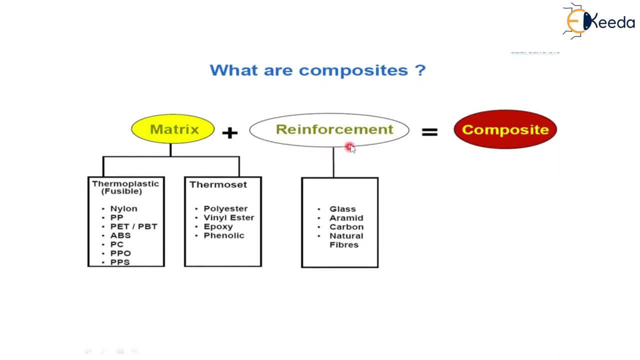 percentage to give the strength for the material we are adding. the second material, that is reinforcement. reinforcement is added reinforcement. maybe any other materials, sometimes glass can be added as a reinforcement- aramid, carbon, natural fibers- so many points, that is, so many materials which can be utilized as a 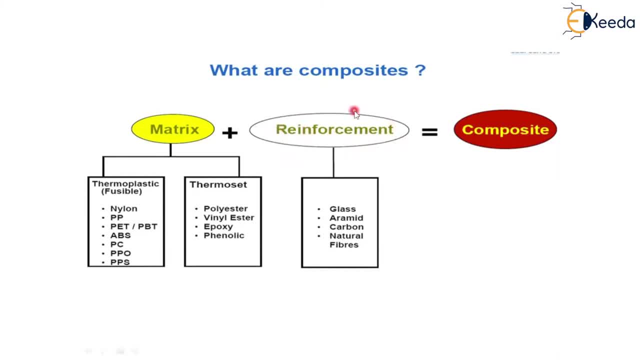 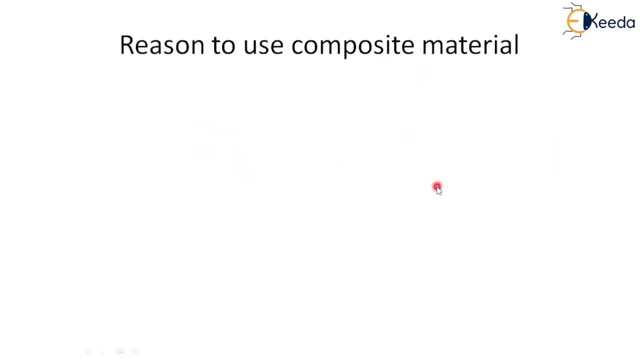 reinforcement. the main purpose or the main property of the reinforcement is to give the strength to the composite material. so let me discuss the reasons why we are going for the composite materials, why the world needs the composite material. see if already pure materials are available, if already alloys are. 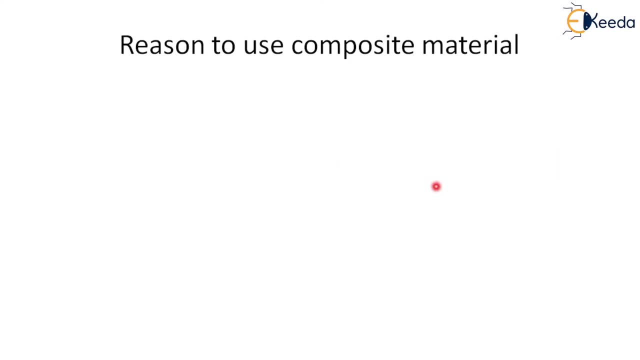 available. why we are going for the composite material. what is the specialty of the composite material? if you see the fastest sentence here? the higher specific strength than the metals, non-metals and even alloys. so this is the point, is the sentence which is very, very attractive. why? 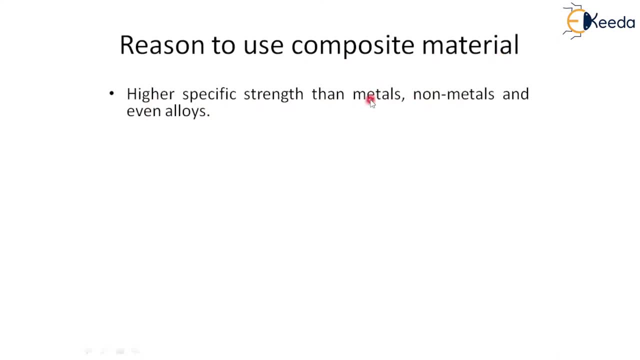 we are utilizing, or why we are going for composite materials. compared to the composite materials, compared to the metals, compared to the non-metals, even per allies rather than the allies, we are now utilizing composite materials and this composite materials having low specific gravity in general and improved stiffness of the material, so that means stiffness of the material is high compared. 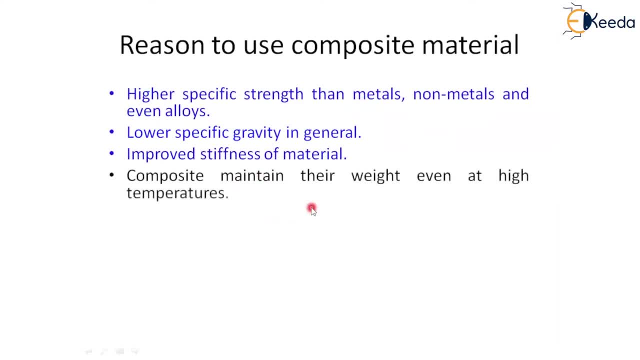 to the other materials and composites maintain their weight even at a higher temperature. that means no change in weight in material loses its weight at higher temperature but composite materials are not going to lose. their strength and toughness is improved and fabrication or production is cheaper for composite material compared to the metals, compared to the non-metals and even alloys. 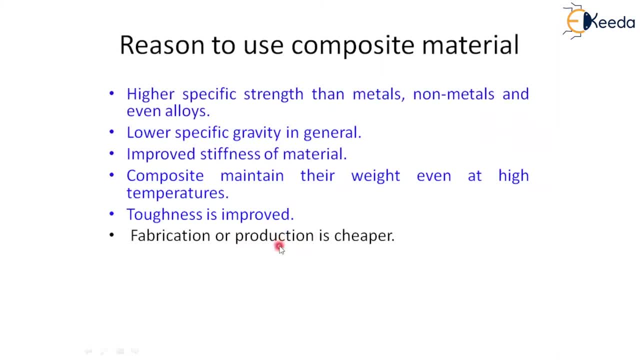 the production process is cheaper for these composite materials and creep and fatigue. creep means time dependent strain occurring, stress. so this particular creep and fatigue strength is better compared to the other material. fatigue means continuous load at successive intervals of time. so this load, this strength is also high in composite materials. that 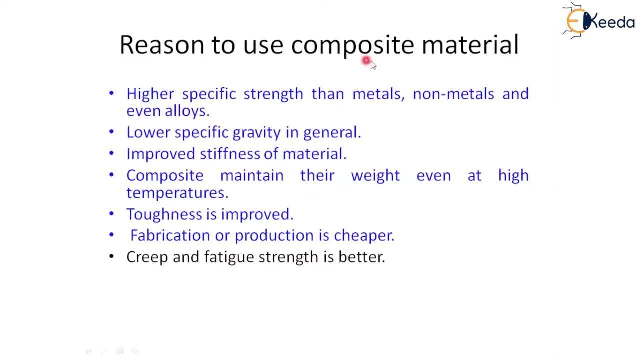 means even if you give the continuous impact on the composite material, it can sustain. so that is the property of the composite material, and controlled electrical conductivity is also possible in composite material, and corrosion and oxidation resistance is the main parameters, which is very, very attractive compared to the metals, compared to the non-metals or even alloys. 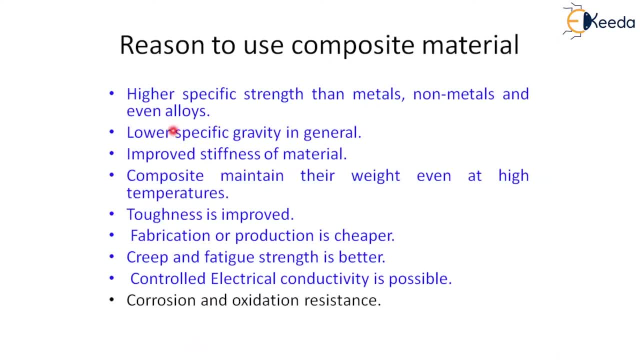 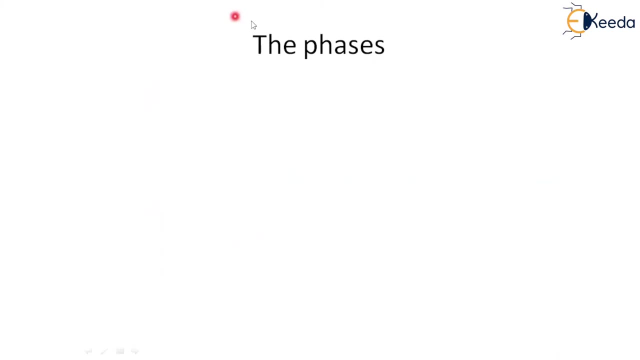 here. this is a corrosion and oxidation resistance that means this composite material can be utilized in all cases. and these are the various reasons why we are going for the composite materials. and now let me discuss the phases, the different phases which are available in composite material. let me discuss the phases, the various phases which are available here now in general. two: 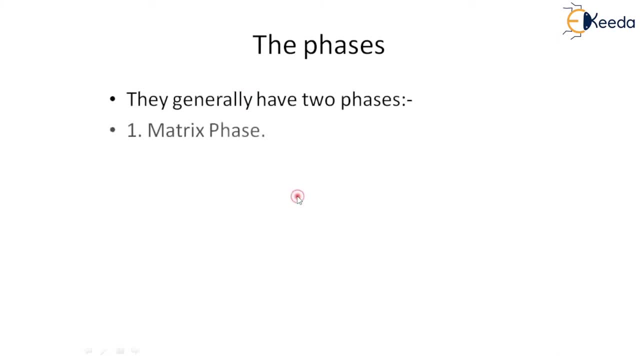 phases are existed here: the matrix phase and dispersion phase. first of all, matrix phase. what do you mean by matrix phase? actually, it is the continuous material constituent of which, which encloses the composite and give its bulk form. so that means the maximum percentage in two materials: the material which is having the 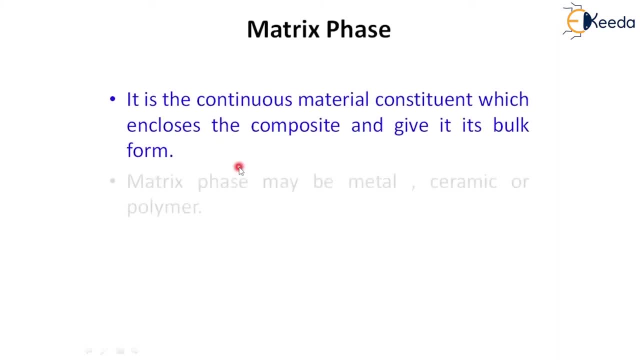 maximum percentage can be represented as a matrix phase, and this phase may be metal or maybe ceramic, maybe polymer. so depends on that, we can call that material as a metal matrix composites and ceramic composites or polymer composites. so this is the main phase in composite material. the main composition of the composite material is: 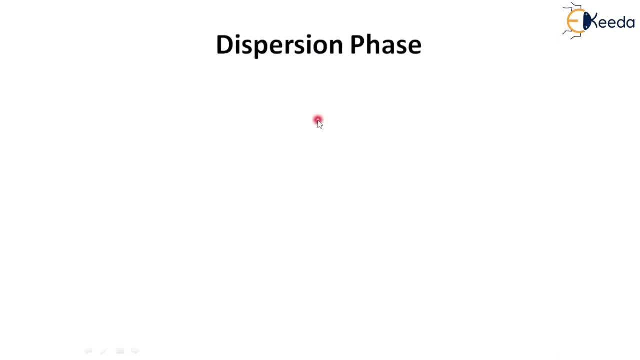 If it is a dispersion phase, that means the second material. the dispersion phase means and consists of here there is a structure constituent which determines the internal structure of the composites. That means the second material, which is represented as a dispersion phase, is induced, or we can say in other words, it is a structure constituent and it will form the internal structure. and this particular dispersion phase is connected to the matrix phase by bonding. 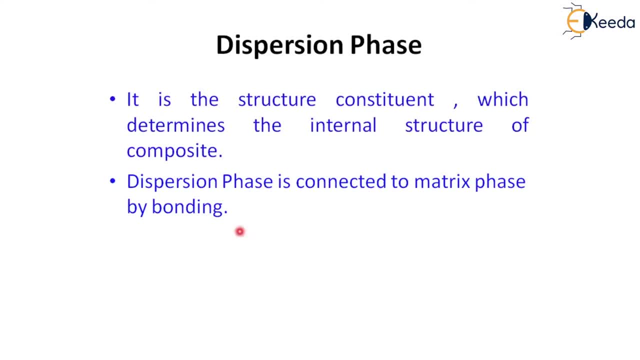 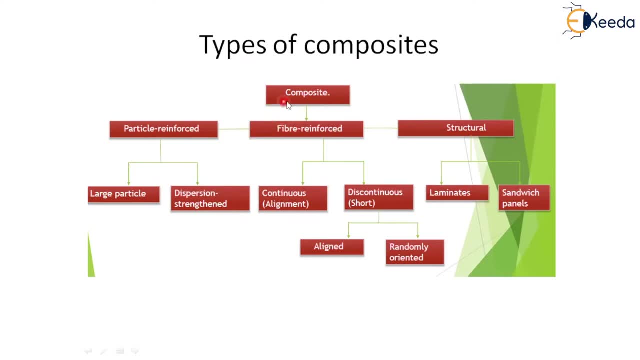 Whatever the bonding, so it is connected to the matrix with the bonding. You can see the types here, the various types of the composite materials. Here this composite material is divided, that is into particle fiber structure. These are the three general composite materials. and particle reinforced composite material is again divided into large dispersion. and fiber is divided into continuous, discontinuous and structural is divided into laminates and sandwich. 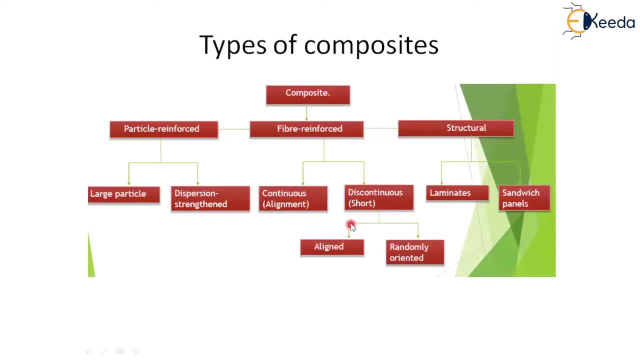 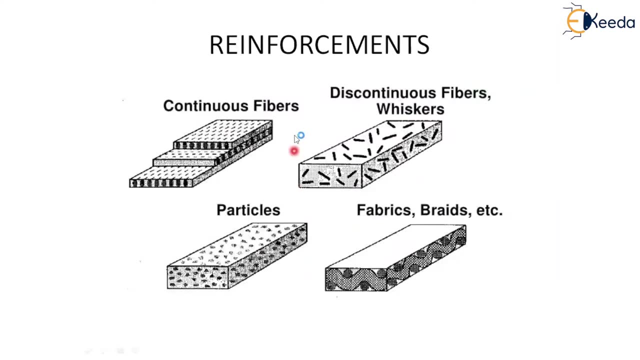 And again discontinuous, is again divided into aligned and randomly oriented. This is the composition, This is the classification of composites and, if you see the reinforcement, the second material in composite materials. so the second material may be continuous, like fibers, and discontinuous fibers like this: 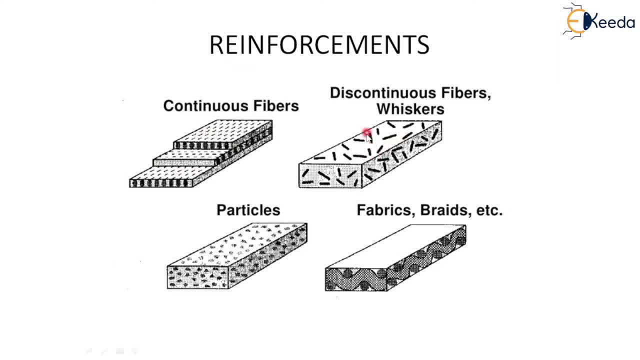 You can see the image here. All these are discontinuous fibers and the second material may be added. in terms of the particles also, You can see here- all these are particles is the matrix and in these matrix the second material is added. So these are the various reinforcement with which we can attain strength. You can see in another image. So this is the fiber reinforced composite material. 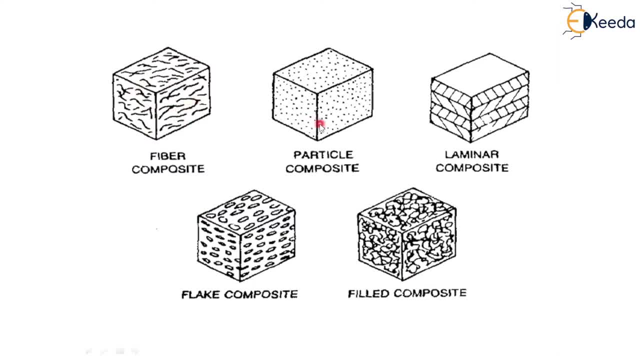 That means in the matrix fiber is added, And here particle composite is a particulate reinforced composite and some laminar. So that means the materials are added layer by layer. You can say: the best example for this laminar is this: laminar is plywood and these are the flakes and sometimes filled composites. So these are the various. 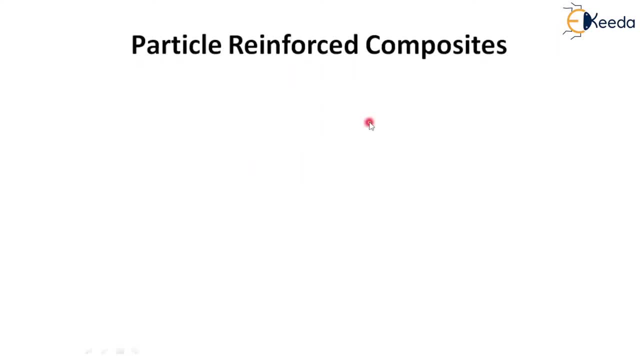 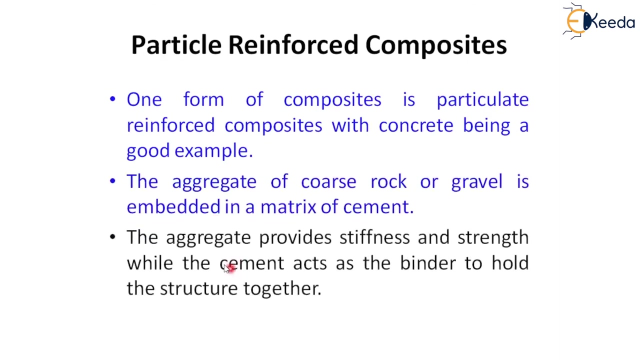 composite material. Suppose: if you see the particulate reinforced composite material, it is actually one form of the composite materials vastly used and particles are acting as a reinforced composites. If you take the example, concrete is a good example and the aggregate- coarse rock or gravel, is embedded in matrix of cement. and if you see the another one, 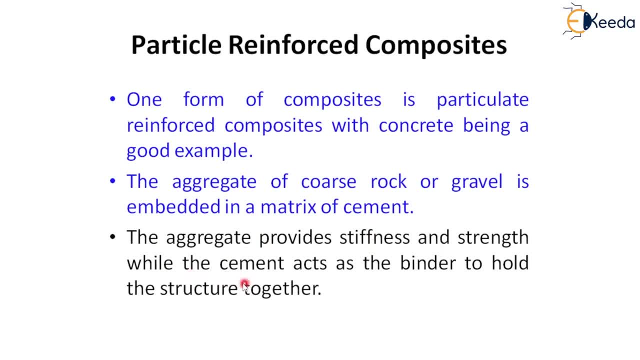 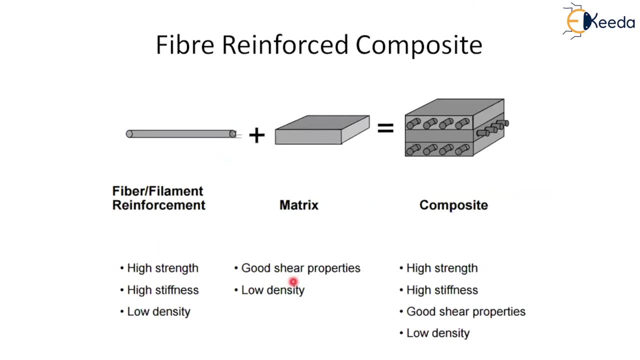 the aggregate provides stiffness and strength, while cement acts as a blinder here. That means any one material has to act as a binder between reinforcement and the matrix. Here this is about the particulate reinforced composite material, and if you see the fiber reinforced here, this is the 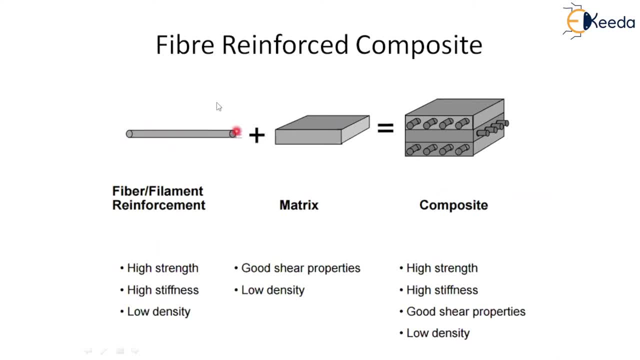 fiber. It is a thread form. The material is in the form of thread or filament, So this acts as a reinforcement. This is a matrix, That means maximum percentage of the material. So if these two are added together, so then it can be represented as a fiber reinforced composite. 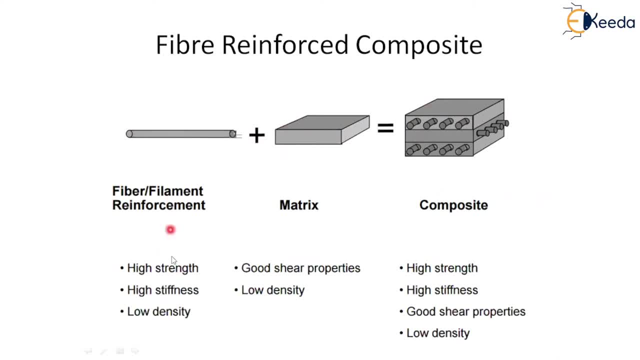 material. So these are the properties of the fiber: high strength, high stiffness and low density- and matrix is having good shear properties, low density, and the composite ultimately by mixing these two. So that means the composite will get both the fiber properties and the matrix properties. 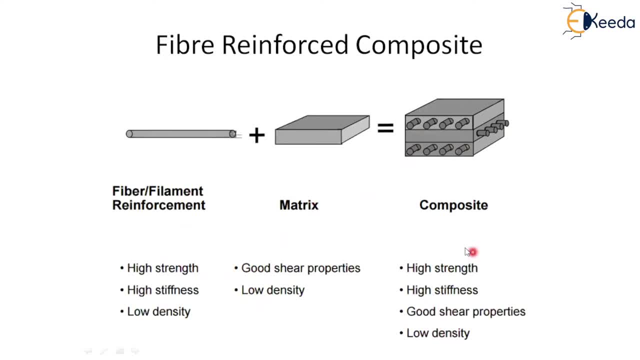 You can see here clearly. it represents the high strength which is actually the reinforced material strength, high stiffness- this is also reinforced strength- and good shear properties and low density. So low density is the matrix property. So by adding together we will get. 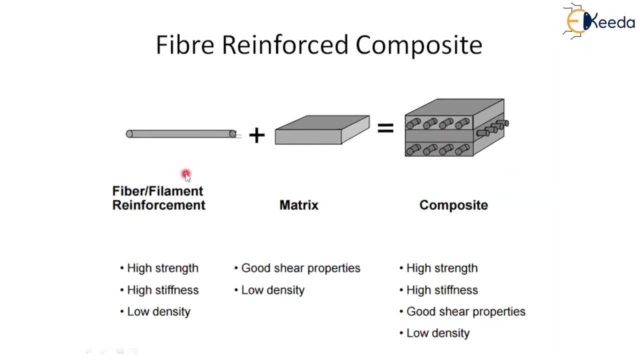 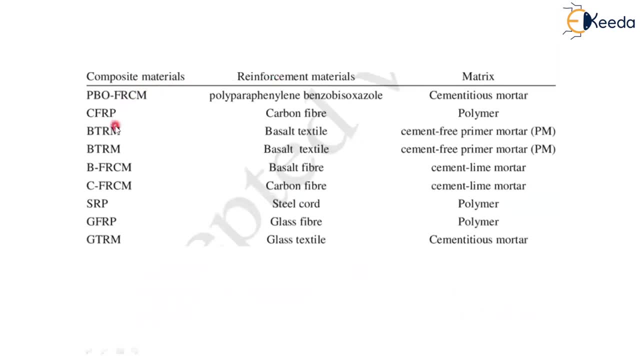 a material in which the combined properties are available of matrix and fiber, And you can see the various features and shortcuts here. This is a carbon fiber reinforced composite material. This is a PBO- polypropylene benzoyl peroxide, And here the basalt is added. here. 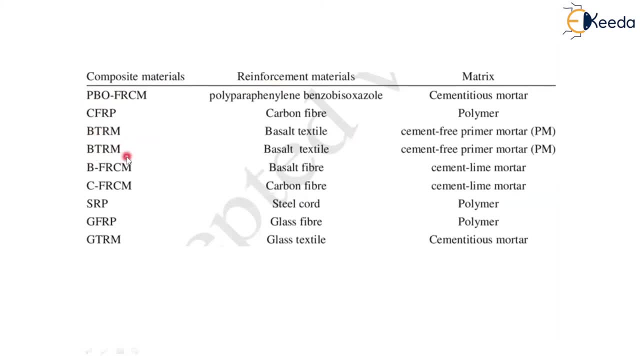 That is the basalt as a reinforcement and here also the same It is that is used in textile industry And B-Phosium. there is a basalt here. Basalt acts as a fiber second material. That means the second material may be added in terms of the fiber And SRB, steel coat and glass.